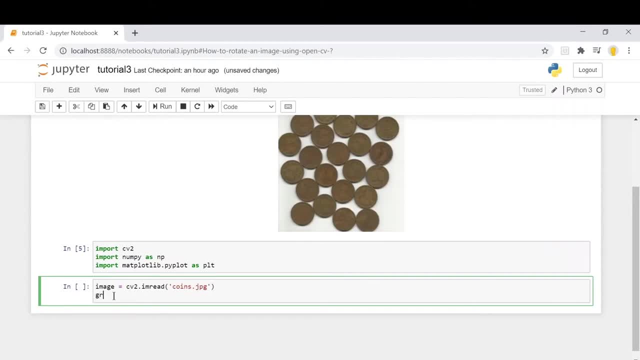 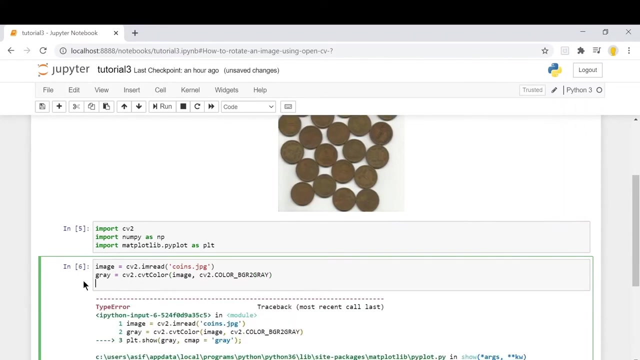 Ok, Now both the images have been saved, Only our image will be using matplotlibspldimso function now, since our image is a grayscale image, so we will be using cmap. equals to gray parameter. 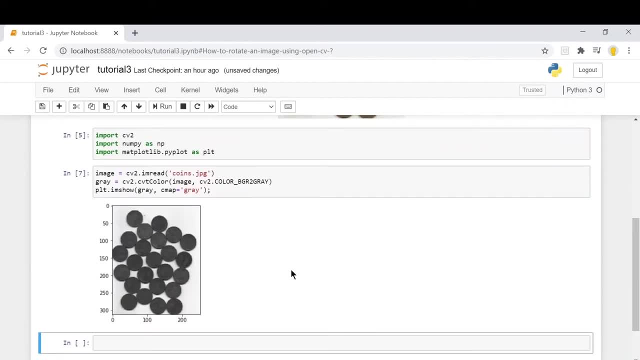 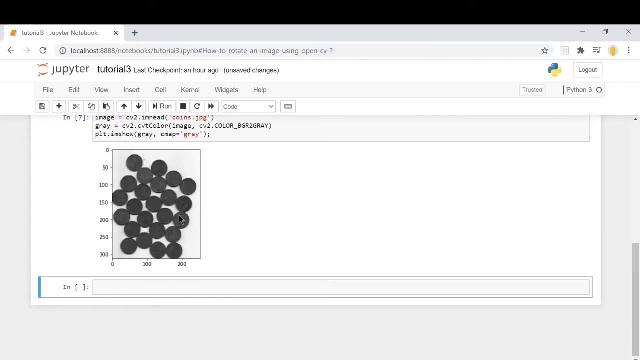 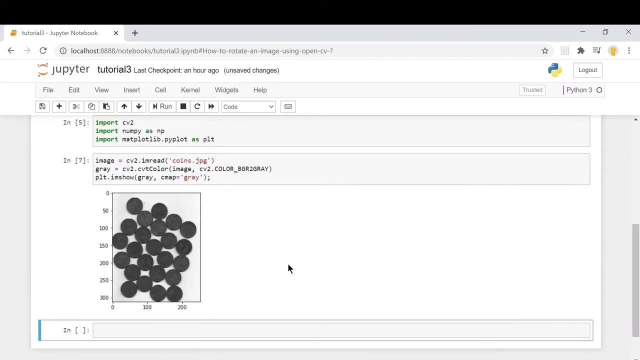 now you can see, we have displayed our image. now, to count the coins in an image, we will have to detect the edges. but before detecting the edges, we will have to make the images blur in order to avoid detecting the noises. so we will be using gaussian blur function. 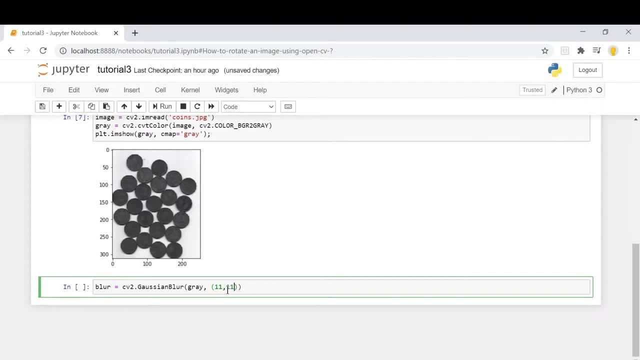 so here the first parameter is nothing but our input image, and the second parameter is the size of the kernel window which will hover over the entire image and calculate the central pixel value using the gaussian algorithm. and this zero value is the standard deviation. so here zero. it will keep this value as zero, so it will calculate the standard deviation on its own. 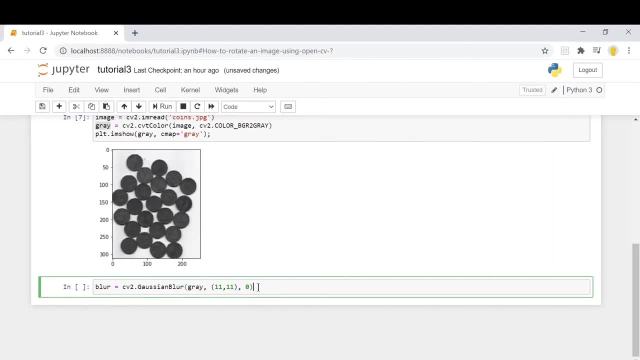 so we don't need to worry about the calculation or standard deviation. so it will increase the size of this kernel, so the image will become more blur. so let's see how our image shows up after making it blur. now lets take a look at the image appear as high. and if we 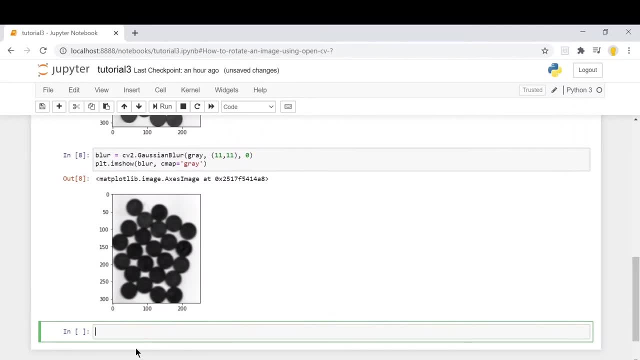 use view. that is. it is here, you can see, we have blurred our image. now we will be using cany eyes detector algorithm for detecting the edges. here, you see, we have blurred our image. now we will be using a cany detector algorithm for detecting the edges. 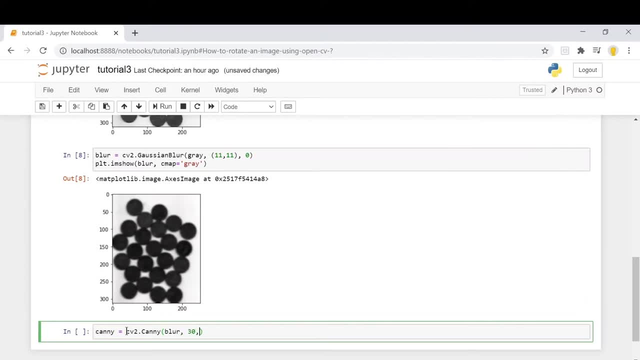 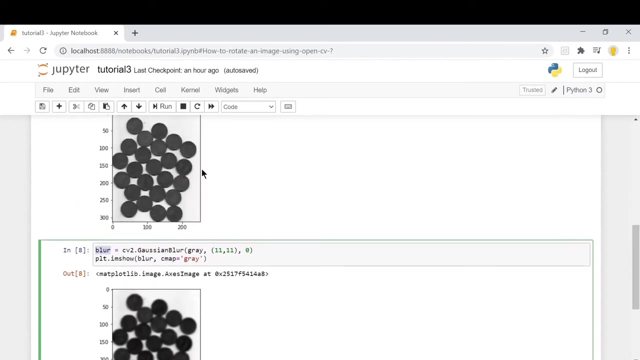 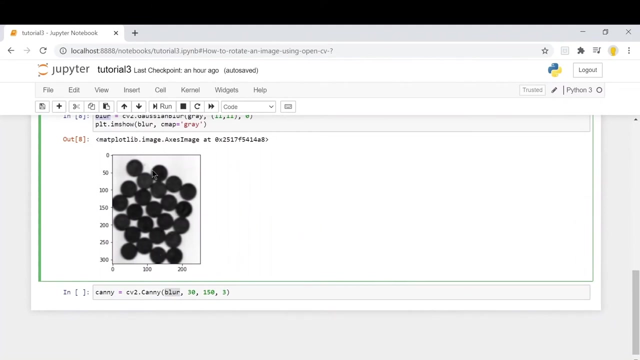 so here the first parameters are input image, which is this one. so we will be using this image and not this called the first image. okay, because we don't want to capture the noise right, we only want to capture the edges of the point. so this is the first parameter. 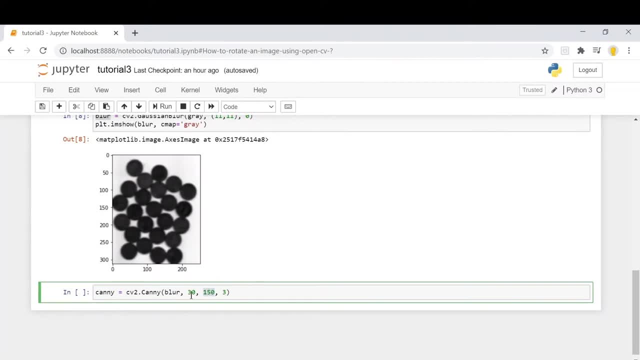 second parameter and the third parameter are is the minimum value in the upper value of the threshold. so a canny detector will calculate the values of the edges and if any edge has a value less than 30 it won't be considered as an edge, and if any edge has a value over one, 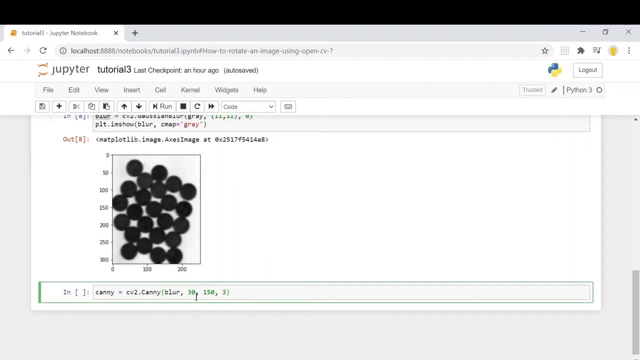 50, it will be counted as a shortage and any value that lies between 30 and 150 will be considered as an edge, depending on if it is connected to the edge which has a value greater than 150. all right, and the third parameter. the fourth parameter is the kernel size of the sobel. 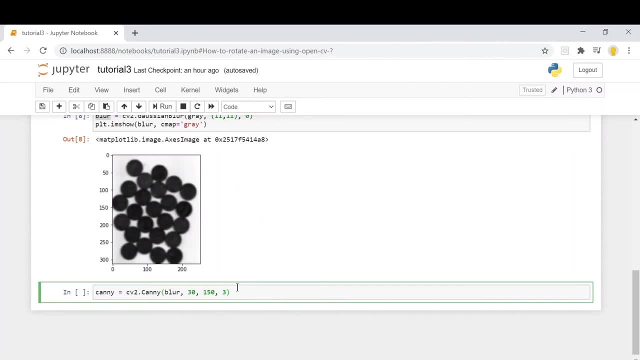 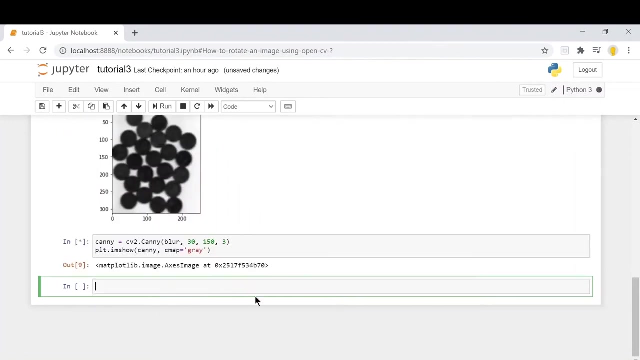 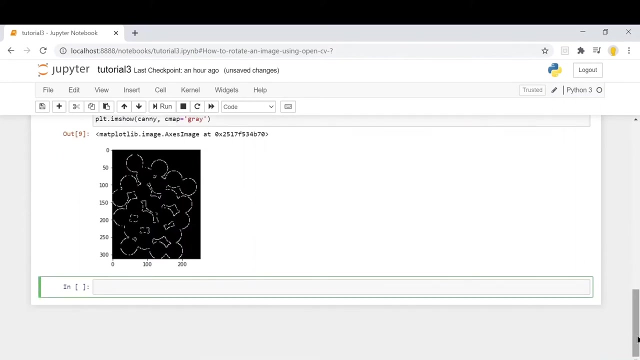 sobel filter which will be calculating the edge. so three is the default value actually. now we'll see what will be the value of this output. so you can see we have successfully detected the edges. now let's proceed further. now you can see that the edges are not connected. 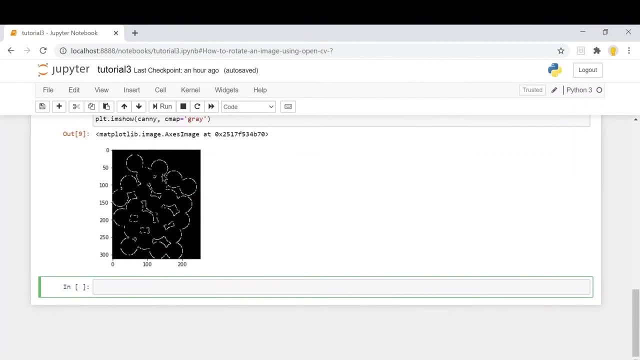 so we need to connect the edges, that is, we have to make the edges thicker and more visible and more connected to each other to fill in the gaps. so we'll be using direct function in cv2. so so, so, so. so no problem now, if you see, the edges are more clear now. 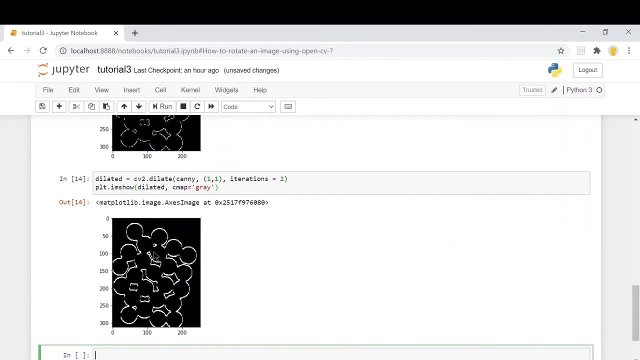 now, if you see, the edges are more clear now. so where this kernel size? and directly it will move this. it will move this kernel across the entire image and and if under that window any white pixel falls, so it will make the other pixel white as well. and we repeat, repeat this process twice, so hence iteration is equal to 2. 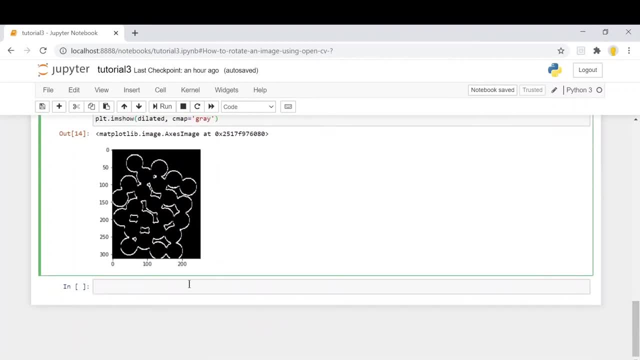 now we can see the edges are more clear now. so now next step is to calculate the contours. so now we find the contours in the image. the first parameter is our input image. second parameter is cv2.retr. external. so so we can see that the contours are more clear. and we can see that the contours are. 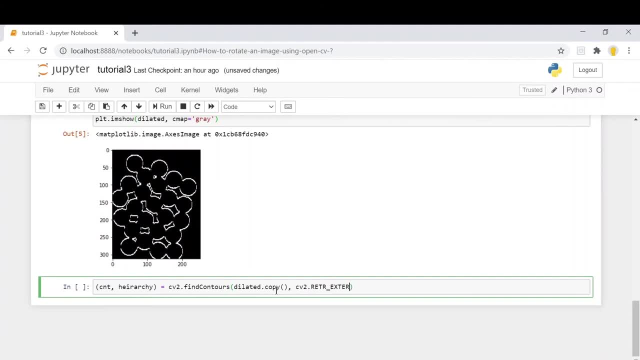 3rd parameter is cv2.ChainApproximal or NULL. we will use NULL. so 2nd parameter: retlExternal means that we will be considering only the external controls and not the internal ones, and chainApproximal is how we will be calculating the contours. it means that we will be considering 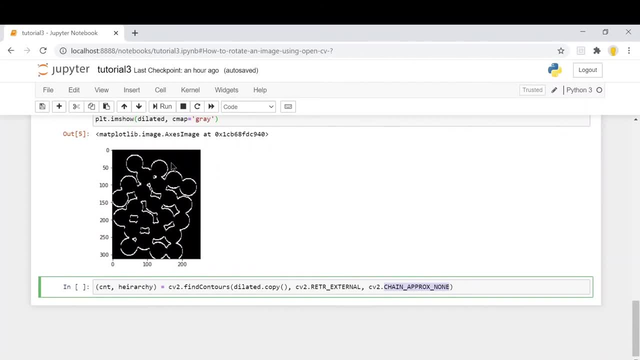 each and every point of the edges to calculate a contour. Now, once our contour has been calculated, we will draw the contours on our image. So, before drawing the contours on our image, we will have to convert our input image into a pgr, into rgb, because cv2 is also an image in bgr format and macroclip is an image in. 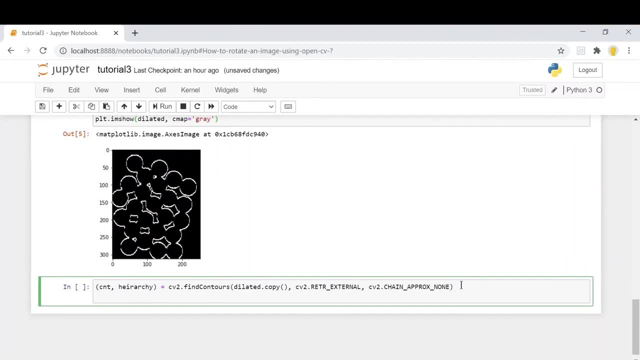 rgb format, so we have to convert our pgr into rgb. If you want to know the difference between pgr and rgb images, you can watch my other videos. Now we will draw the controls on our image. First parameter will be our input image. second parameter will be the contours. third parameter: 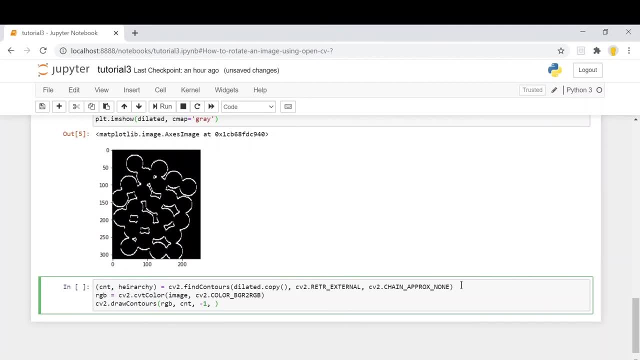 will be how many contours we have to draw. So we will want to draw all the contours. and fourth parameter will be the color of the contours. So we will consider green color. and the last parameter is thickness. So let's draw, Let's display our image. pltemissor function. 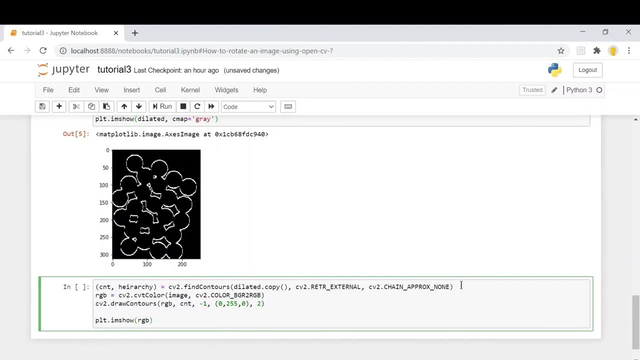 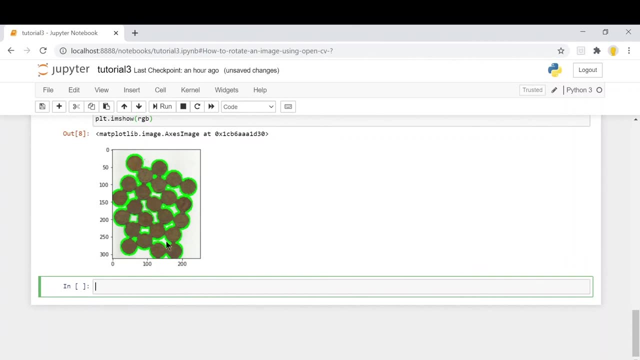 So we won't be using cmap now over here. So here you can see we have drawn the contours. So now let's count the points in the image. I will just write here a simple statement: points in the image 24.. So we have counted 24 points in this image. 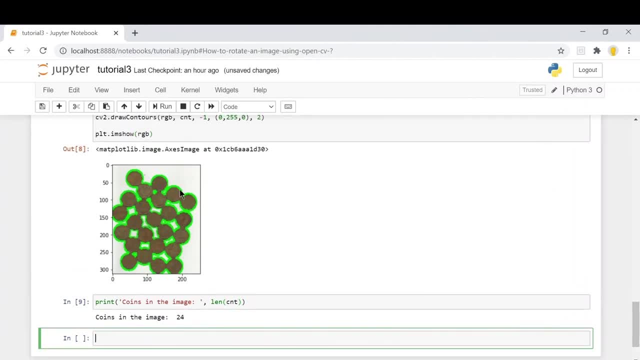 So let's verify: 1,, 2,, 3,, 4,, 5,, 6,, 7,, 8,, 9,, 10,, 11,, 12,, 13,, 14,, 15,, 16,, 17,, 18,, 19,, 20,, 21,, 22,, 23,, 24.. 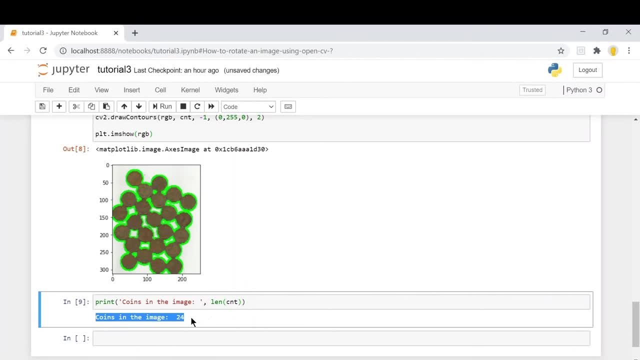 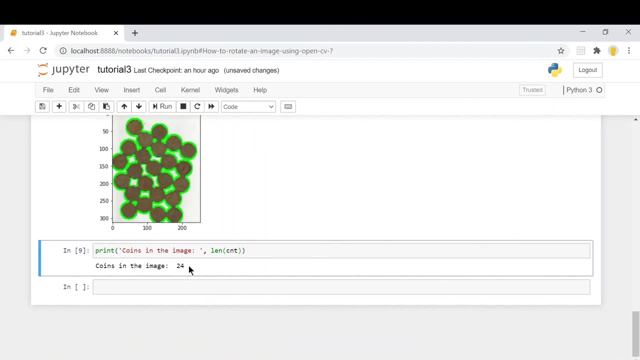 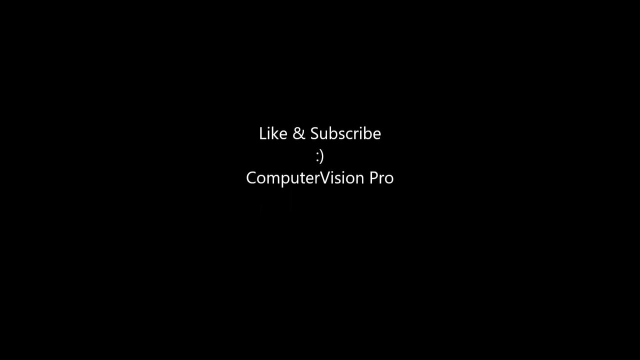 So we have successfully counted right number of points in the image. I hope you found this video helpful. Don't forget to subscribe. Thank you very much. . . . . . . .